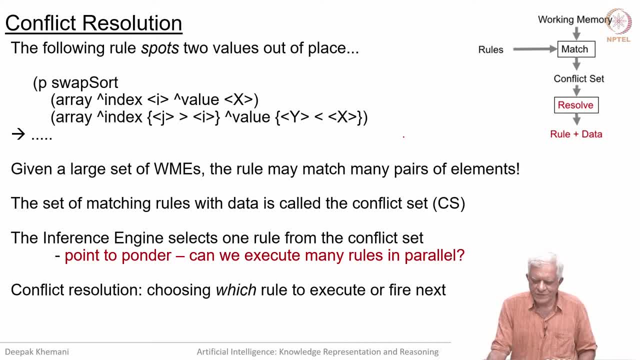 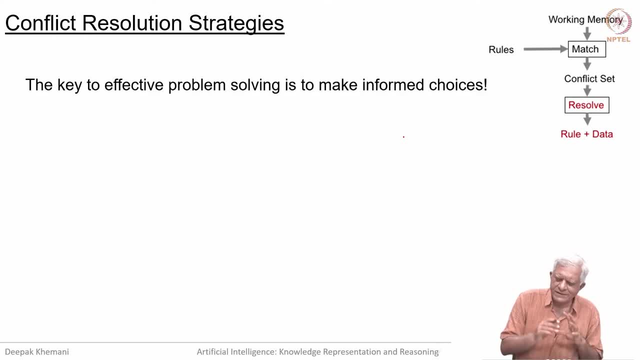 called the conflict resolution task. So let us see what are the kind of strategies that we can implement for conflict resolution. Given that, at any given point, a problem solver may be faced with many choices, the key to effective problem solving is to be making 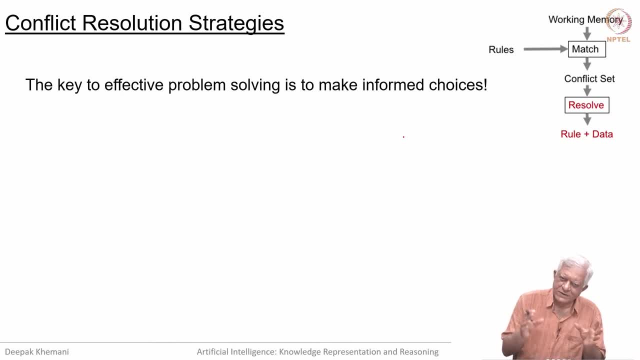 informed decisions about which choice to make, or making informed choices essentially. If you have studied heuristic search algorithms like best first search or A star, you would know that we have a notion of a heuristic function which looks at all the choices and gives them a value and says: then you can say: I will choose the choice with the smallest. 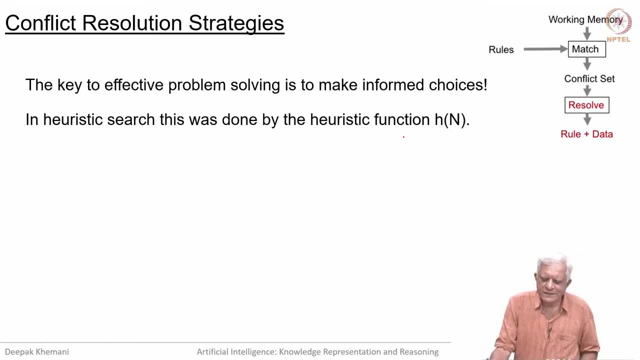 value, and that value is a heuristic function. And that is what we do when we are looking at search essentially In rule based systems. rules encapsulate the knowledge gleaned from search essentially, And then we want to simply say all the rules that are applicable, which? 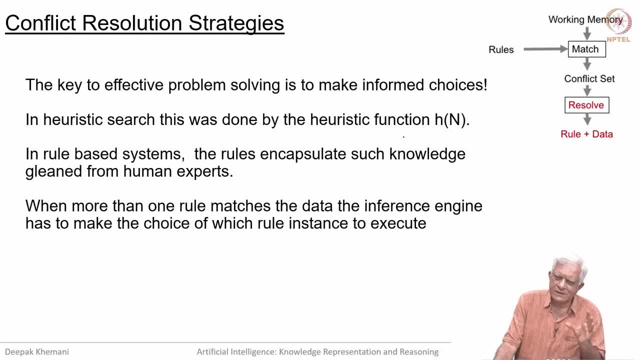 one to fire next. When one more than one rule matches the data, the inference engine has to make a choice as to which instance to execute next. It is a little bit analogous to which candidate to inspect next in search, essentially, And we will look at some conflict resolution. 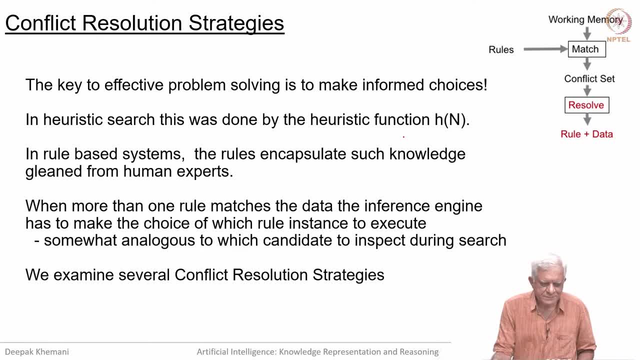 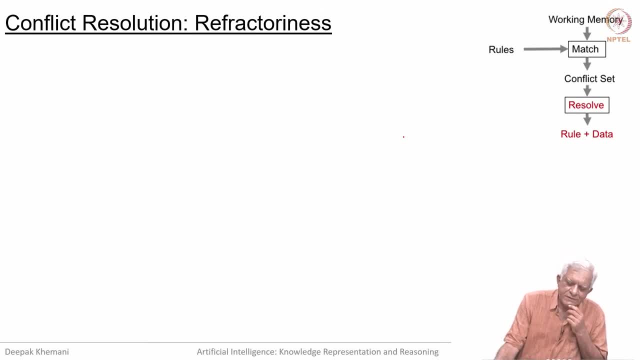 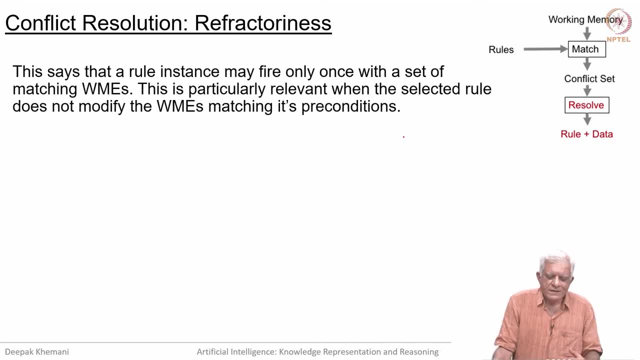 strategies that are popular. So the first strategy, which is necessary in fact, is called refractoriness. It says that a rule instance may fire only once with a set of matching working memory elements. That okay, you have found this rule instance, it matches this piece of data and you can. 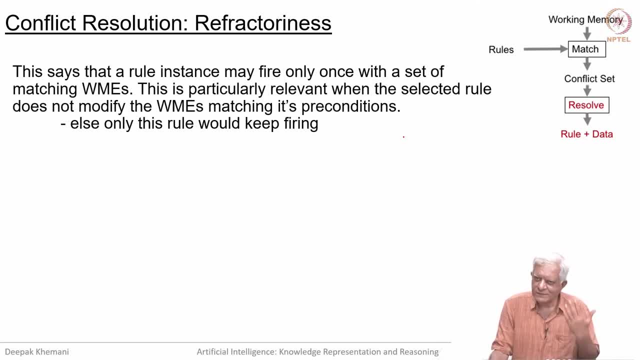 fire it, but you cannot keep firing the same rule again and again with the same piece of data. In fact, the actions of the rule do not have anything which is deleting from the working memory element. If you are not deleting anything from the working memory element, even though 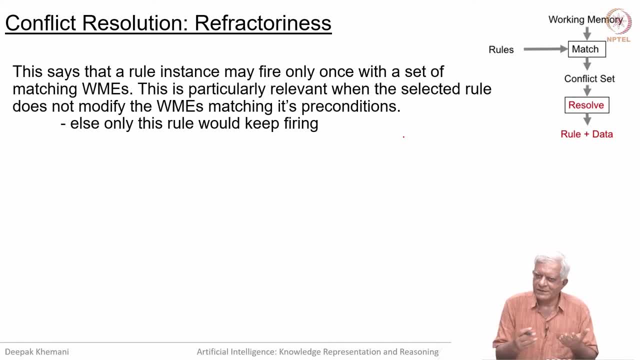 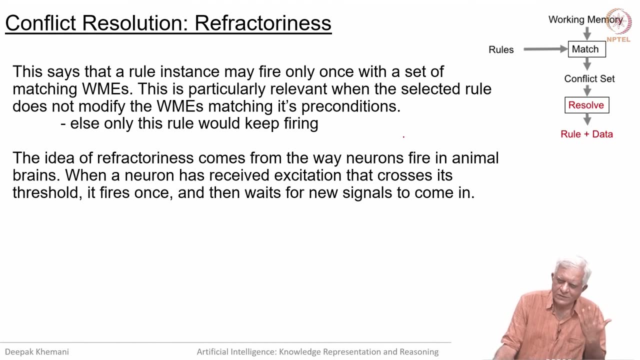 the rule has fired, it would still match again. Refractoriness says that this is not allowed. Otherwise, there is always the danger that that one single rule will keep firing all the time. The idea of refractoriness comes from the way neurons fire in our brains, So 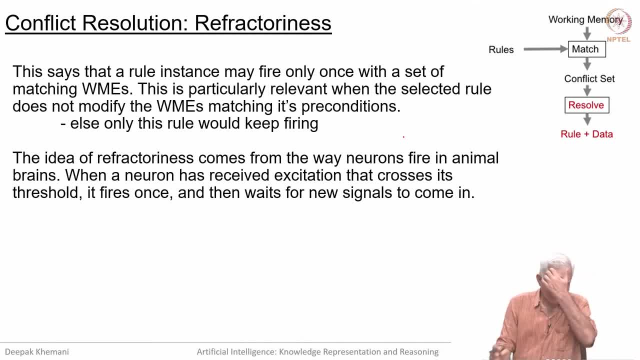 that is why, because when the the way that neurons fire, if you have looked at neuron networks, is that the neuron gets inputs from many other neurons And there is some sort of a function built inside this which will look at which is some of the inputs and you 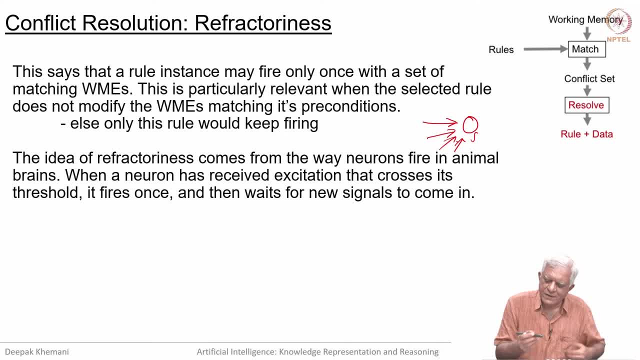 know, there will be some thresholding and maybe some sigmoid function or something like that, So one that, as they call, in terms of neural network, as the exception of this. as the excitation level goes up, the neuron will fire and it will create its own impulse, which 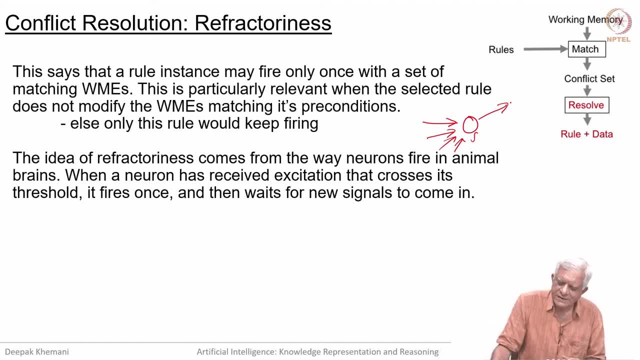 will travel down the action of the neuron. essentially, Now, what happens is that in in physical brains these excitation is in terms of chemical, electrical signals, So once it is used up, then the neuron has to wait again for it to get built. 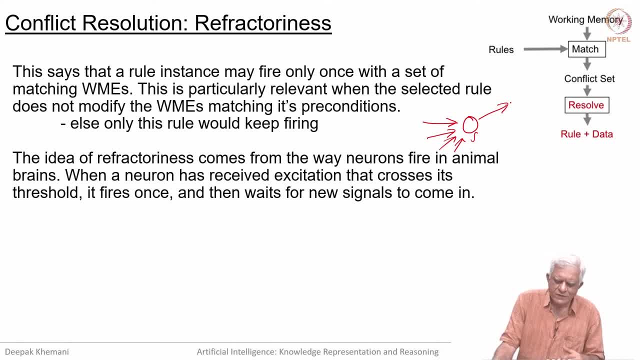 up again. So it happens naturally there. So when a neuron has received excitation that crosses the threshold, it fires once and then waits for new signals to come in. essentially So, then the name refractoriness comes from there, In terms of rule based systems. 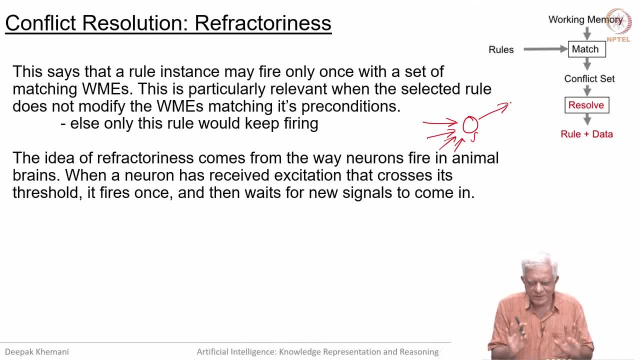 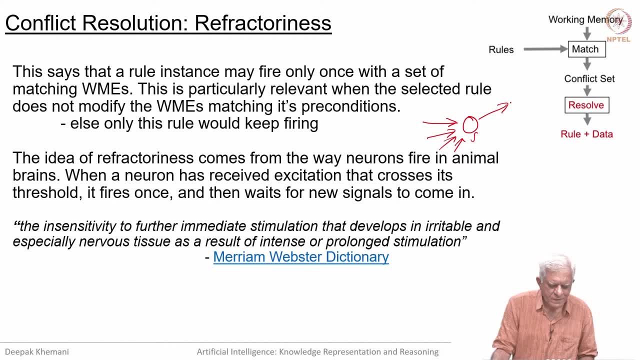 it means that a rule instance with matching data should fire only once. We will see that that happens naturally in the implementation that we will talk about. So this is the definition of refractoriness. So refractoriness from this Merriam-Webster dictionary, the insensitivity to further immediate. 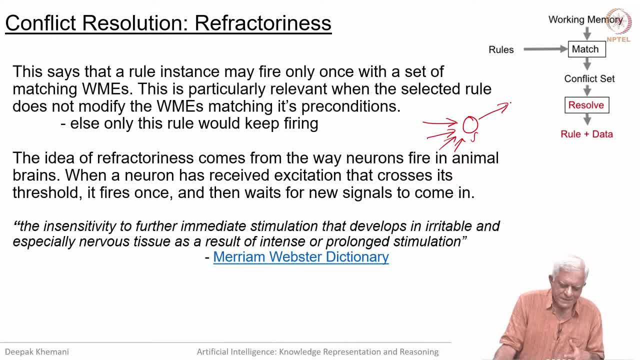 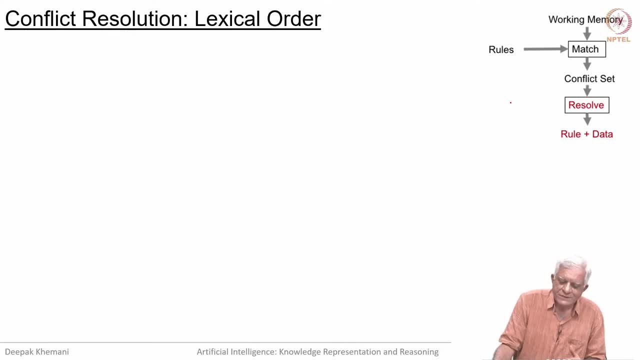 stimulation that develops in irritable and especially nervous tissue as a result of intense and prolonged stimulation. As we will see, we will look at this algorithm called the rate algorithm, and refractoriness will happen naturally in this algorithm. So here is the second conflicts resolution strategy. This is called lexical order. essentially, 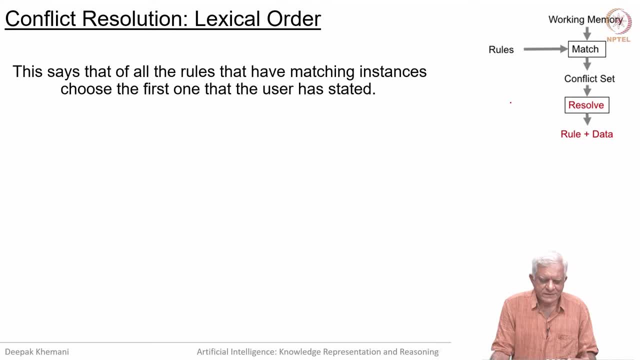 It says that of all the rules that have matching instances, choose the first one that the user has stated. So user has written the rules in some order. choose the first one that matches. If a rule has multiple instances that match with different data, then choose the instance. 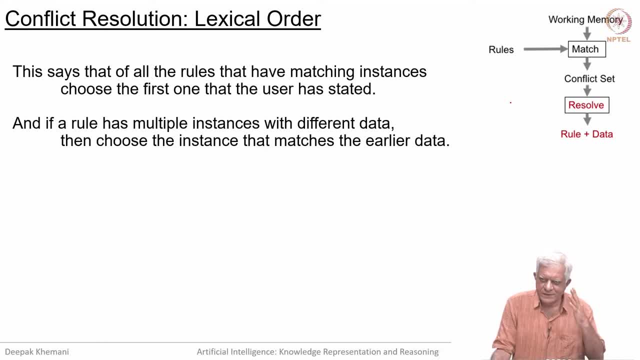 that matches the earlier data, because the data also is an ordered set. The strategy, this strategy, This strategy places the owners of the choice on the user. The user is more like a programmer and we have seen that this is the kind of strategy that prologue uses The prologue. 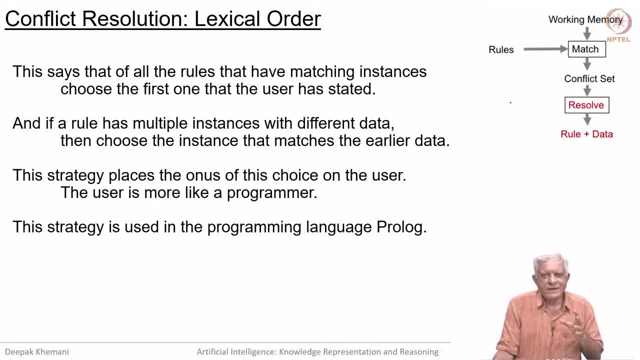 says that I will look at all your rules in the order that you have written and the facts are also written inside that same file and they are also written in a particular order. So prologue always looks at things in lexical order. So I have mentioned it is a couple. 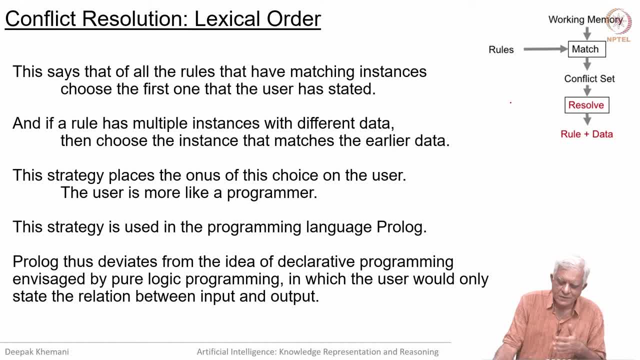 of times that real prologue As opposed to prologue. the real prologue is the one that is called pure prologue. Real prologue deviates from the idea of pure declarative programming, where I would only have to state the rules and the facts and it would somehow solve the 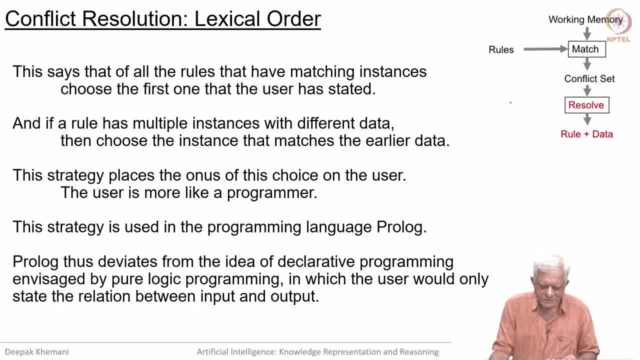 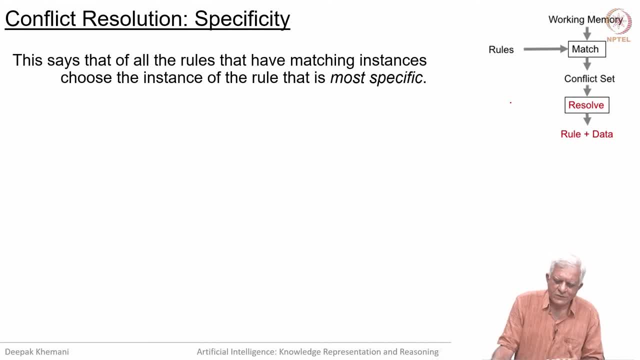 problem for me. In prologue, the order in which you state the rules is also important, which is a bit more like programming. So here is another strategy called specificity. This says that of all the rules that have matching instances, choose the instance of. 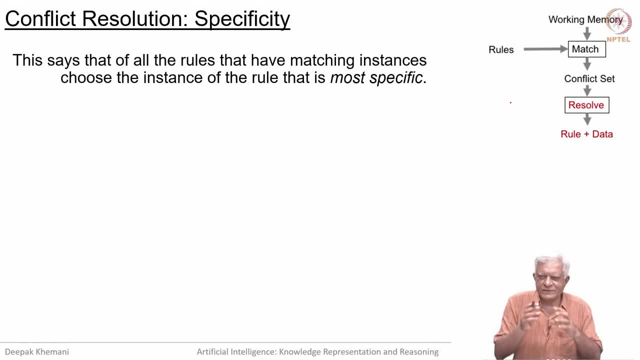 the rule that is most specific. So if one rule is specific, that means that all the rules that have matching instances choose the instance of the rule that is most specific. So if one rule is specific, then one rule matches two pieces of data, another rule matches five pieces of data, then choose. 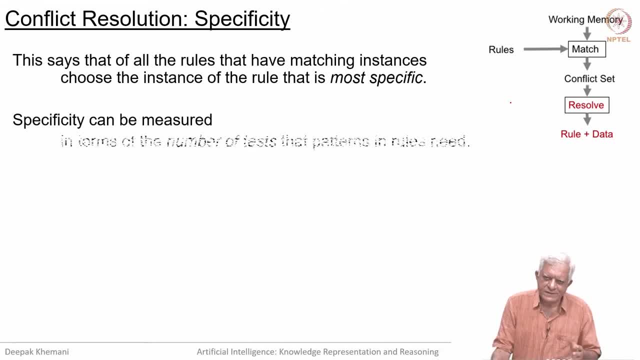 the one which matches more data. It is more specific. As you will see, specificity can be measured in terms of the number of tests that the pattern in the rule, that the rules need. So if you look at the swap program that we saw, it does some tests, that there is one. 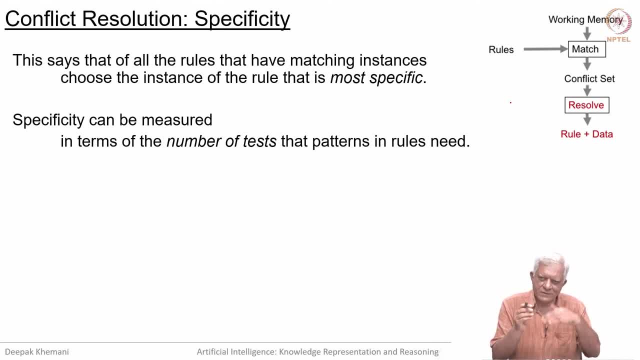 element whose value is this thing. there is another element whose index is greater but whose value is smaller. So it is doing this thing. You can count how many tests it is doing and based on that you can decide which rule is more specific, which instance of the rule is more specific. 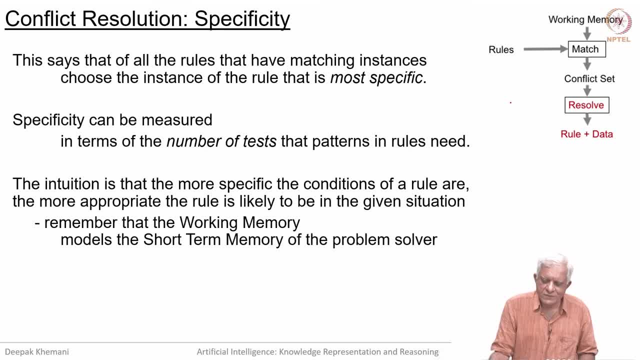 The intuition is that the more specific the conditions of a rule are, the more appropriate the rule is likely to be in a given situation. That is an intuition that we often use. Remember that the working memory models, the short term memory of the problem solver and rules constitute. 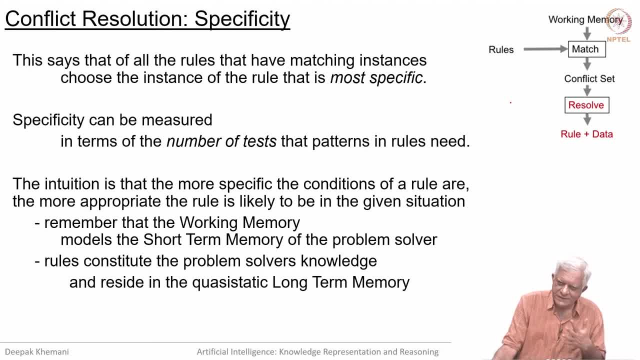 the problems: long term memory. So this is the idea which you see on the quasi-static long term memory. So I am saying quasi-static because you know you are allowed to change rules, of course, but in general when you have built a rule based system it will be kind of constant. 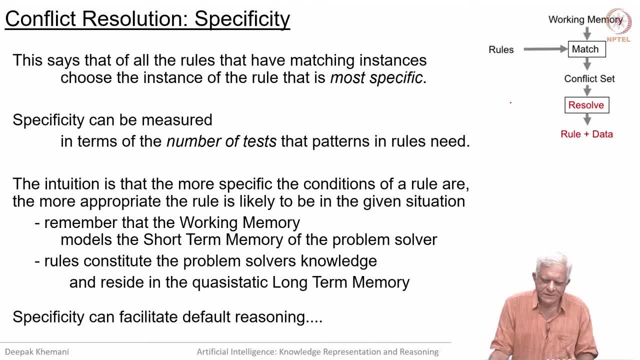 Specificity. choosing this specificity as a conflict resolution strategy can facilitate default reasoning. What is default reasoning? If you know some things, then you make an inference. if you know more things, then may be you make another inference and you do the default only when you do not know the other stuff. essentially, if you know more specific, 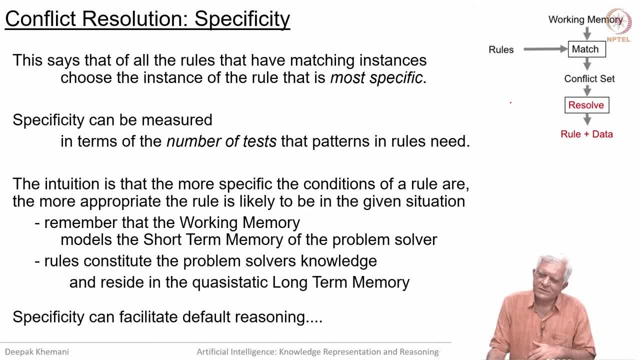 things, then you take the default action. essentially So, the default action is that, for example, I will make a cup of tea at 5 o clock, but then if something happens- and you know, maybe I have to attend to something and some other facts come into play- then I may have a different. 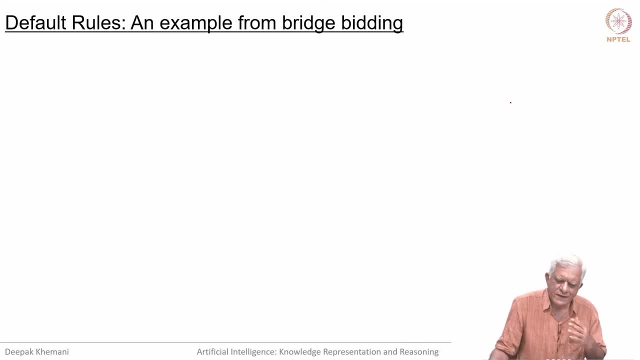 action essentially. So here is an example from the game of contract bids, which I hope all of you will learn at some time, and this is from the bidding phase of the game. So in bidding phase, people are. it is like an auction that is happening and 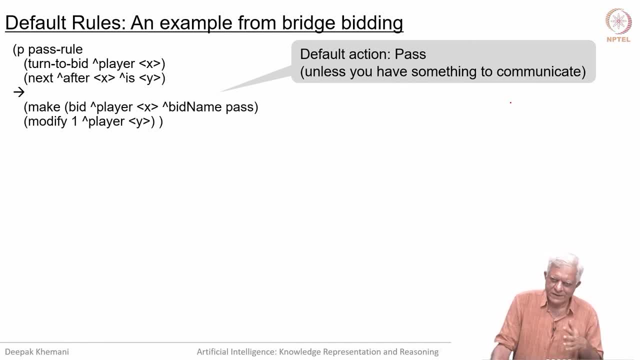 you are making bids essentially. So I do not want to get into the game. that would take up too much time here, but I just want to. I will give you some instance of rules where specificity would be used to take actions when you know more specific information. but if you do not have that information, then you 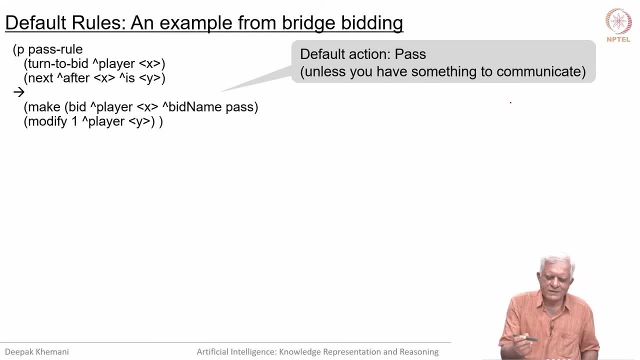 just use a default rule. So here is a default rule which says that unless you have good cards, for example, you just pass, and the default rule simply says that there is a player x, it is his turn to or her turn to bid and the next player to bid will be after. that would. 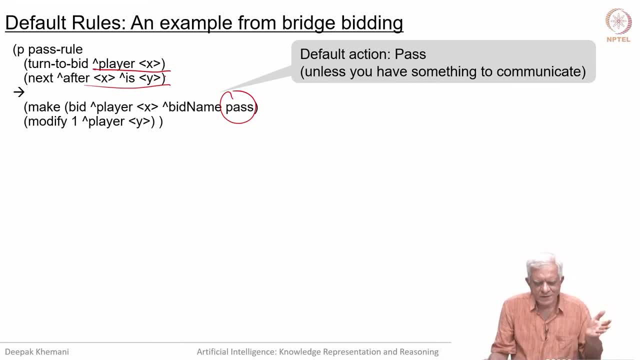 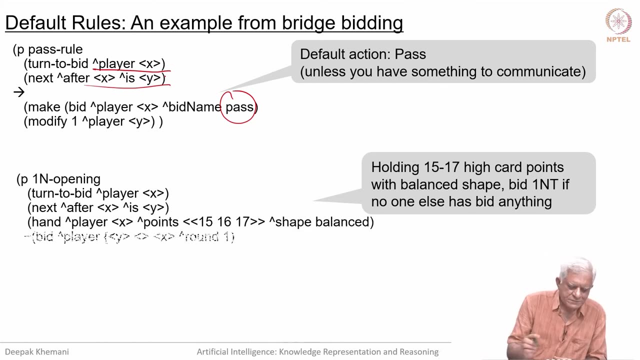 be y essentially. So it is your turn to bid. after you, you would bid and then the default thing is pass. You know, if you do not have some good cards, then you would pass, but if you had good cards then you. that data would be stored in the working memory somewhere, So you can see. 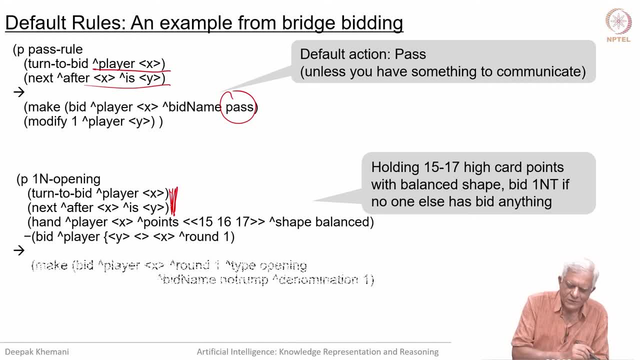 that the first two rules patterns are the same here as in the default rule. but there is something else given here, So you do not have to get into the details. that it is that let us say there is something called high cut points. that bridge say bridge players. 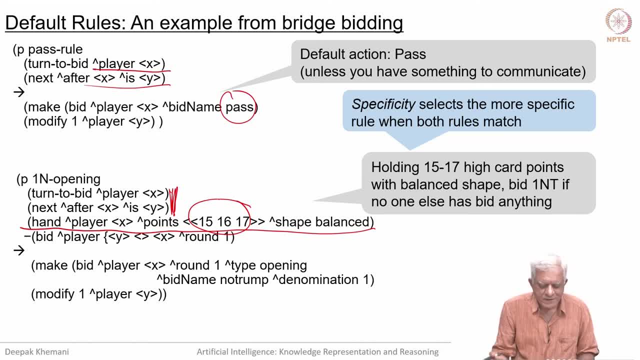 use. So if you have 15 or 16 or 17 high cut points and if the shape of your hand is balanced- by this we mean how many hearts you have, how many spades you have, how many clubs you have, how many diamonds you have, If the distribution is balanced. so there are certain things which 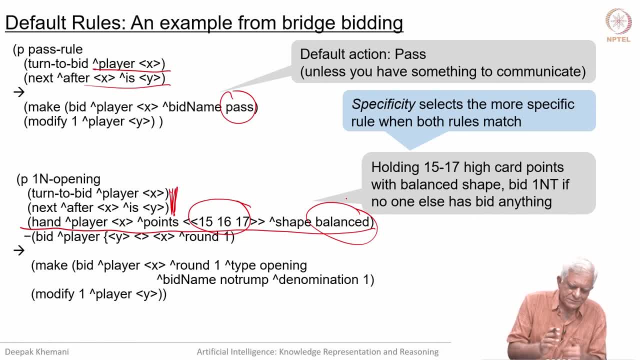 are balanced. there are some certain things which are not. Then you make this bid, which is an opening bid. its bid name is notram and its denomination is 1.. So bridge players would recognize this as saying that if you have 15 to 17 high cut points and you have 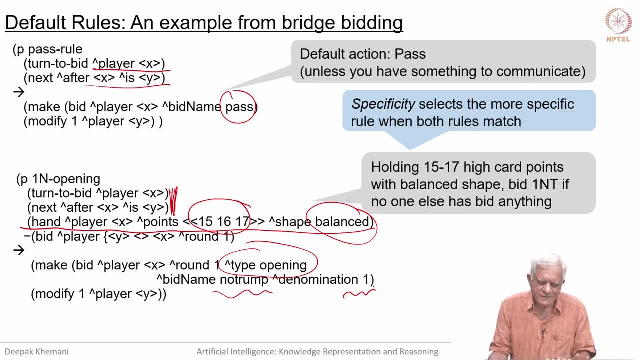 a balanced hand, then you open one notram. If you do not have all this stuff, then you just pass. essentially, Of course there are other bids for making other patterns of making other opening bids. So in general, of course you would choose the most specific. 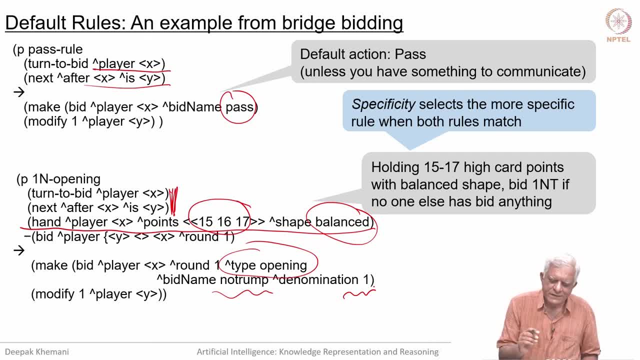 rule instance, and you do not have to worry about whether my program will pass by mystic, as long as you specify that the conflict resolution strategy is specificity. Always choose the more specific rule and if you cannot find a more specific rule, then go to the default rule. We will look at default reasoning again As an exercise. just write. 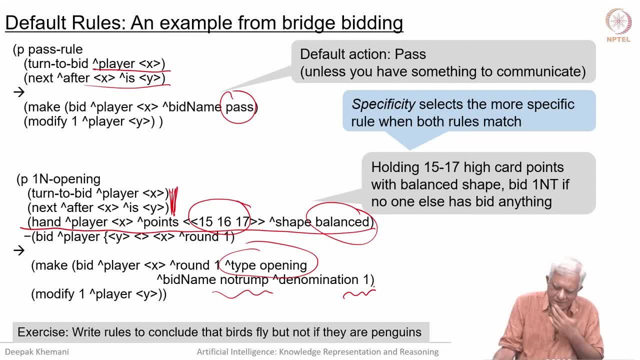 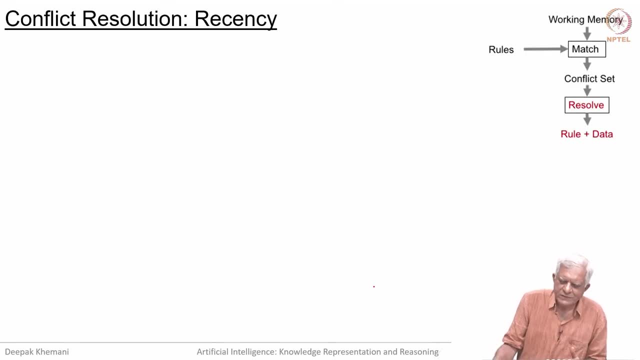 this two rules. one says that birds fly and the other says that if you are a bird and you are a penguin, then you do not fly essentially. Then you can see the specificity would help essentially. So one more strategy that we often use is: 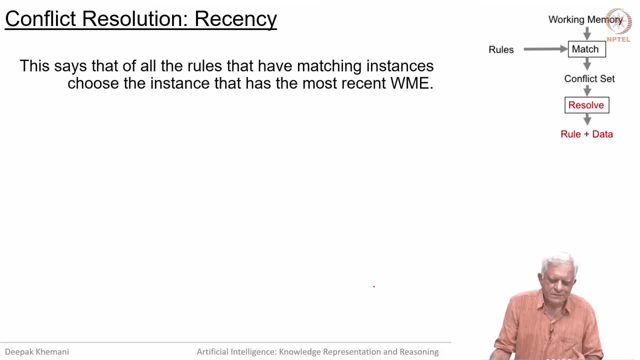 called recency and recency says there are all the rules that have matching instances. choose the instance that matches the most recent working memory element. So remember, the working memory elements have time stamps and you have, let us say, 15 rules in your conflict set and all of them matching different working memory elements. It says: choose the one which. 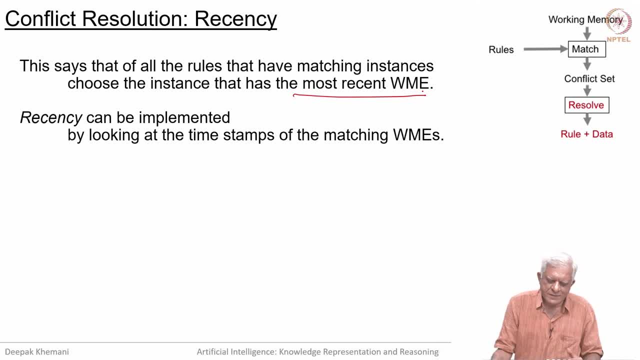 has the highest recency. It can be implemented by looking at the time stamps of the working memory elements, but we will see that there is a simpler way of doing it when we when we implement this algorithm called the rate, net Or rate algorithm. The intuition behind using recency is that when a problem solver adds 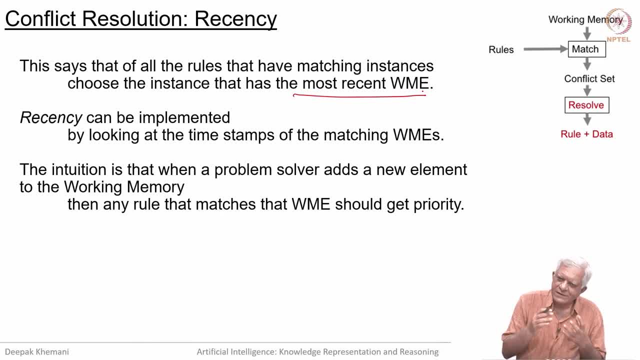 a new element to the working memory, then maybe you want to do something with that working memory element. So there is another rule which matches this. then maybe that rule makes sense to be. it makes sense to use that rule now. So in some sense you want to maintain a chain of thought. You are making a sequence of inferences. 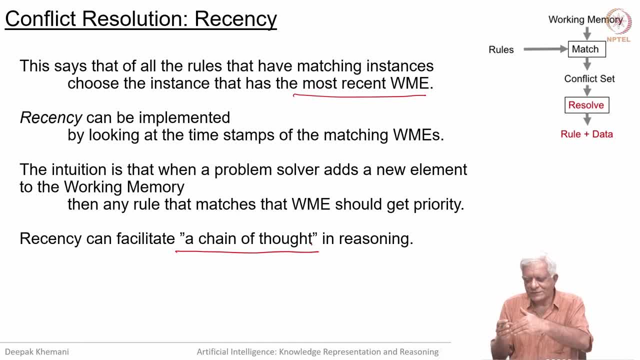 that if this is true, then this is true. and now, if that is true, then something else is true. So, if there is a rule which is looking at that, then give reference to that. So recency will allow you to maintain a chain of thought. Of course, you can maintain the conflict set. 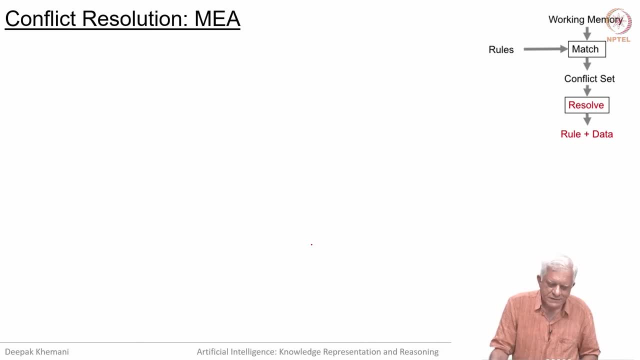 as a priority queue sorted on the recency for each rule, which means the recency of the highest working memory element in that rule. The offside language gave us a conflict resolution strategy called mean sense analysis, MEA, based on the problem solving strategy espoused by. 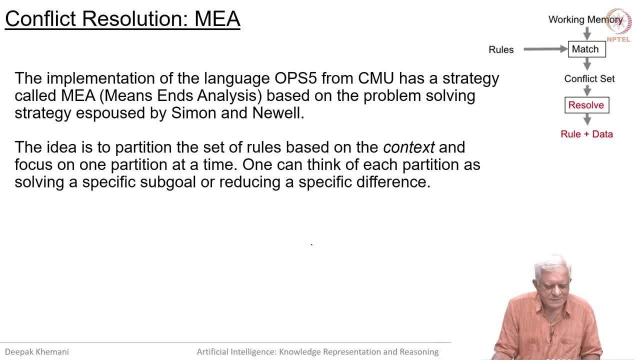 Simon and Newell, who did a lot of work on human problem solving. So the idea is to partition the set of rules on the context- These set of rules apply in this context, this set of rules apply in this context, and so on- and focus on one partition at the time. 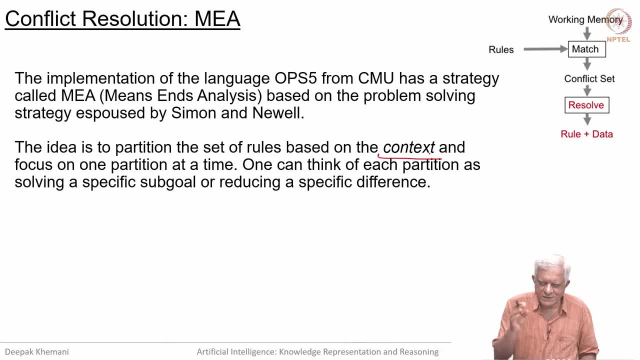 One can think of each partition as solving some specific sub goal or reducing some specific difference is the term that Newell and Simon spoke about. The context is set by the first pattern in the rule. essentially So, in their strategy they first looked at the first pattern. 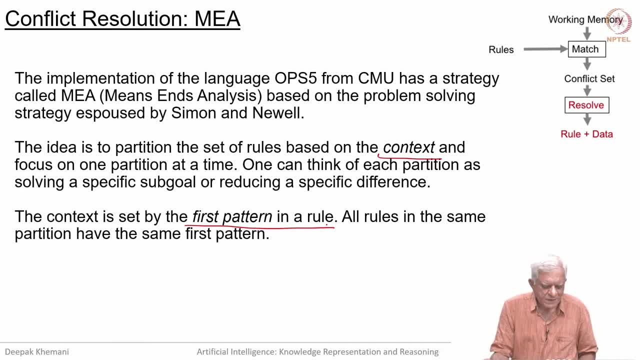 in the rule and then looked at the rest of the rules. All this rules in the same partition have the same first pattern, So its context is do activity x, Context is do activity y, as the case may be, and all rules which are concerned with activity.